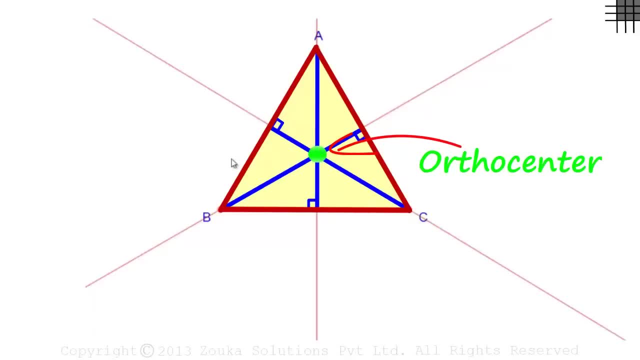 meet at the orthocenter. It is the orthocenter which lies inside the triangle. Does the orthocenter always lie inside the triangle? Let's move vertex A towards the left to form a right angle at B. Now it gets interesting. 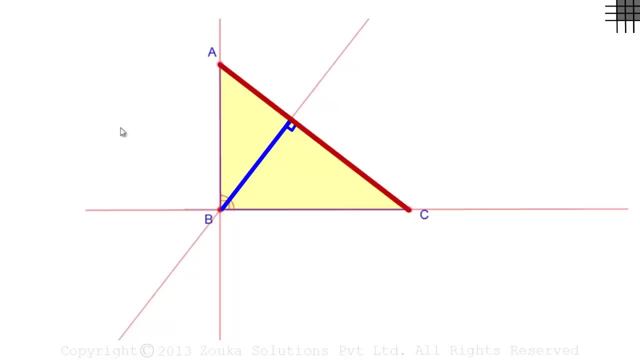 This is the altitude from vertex B to the opposite side AC. But what about the other two altitudes? Where does the orthocenter lie? This segment from vertex A to BC is one of the altitudes. Where does the orthocenter lie? 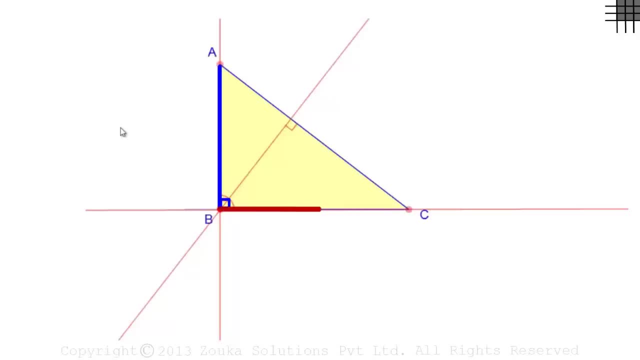 This altitude does not lie in between B and C, it lies on point B And this segment is the altitude from vertex C to segment AB And again it meets segment AB at point B. All the three altitudes meet at point B In a right angle triangle. the vertex at the right angle will be the orthocenter. 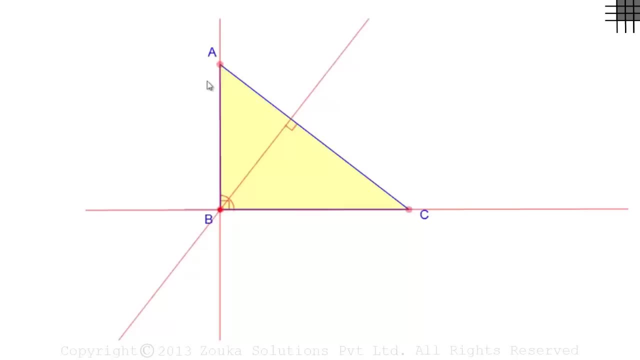 Let's make it even more interesting. We move vertex A leftwards to make angle B obtuse. This segment is an altitude from vertex B to side AC. But to drop a perpendicular from vertex A to a segment BC we have to extend CB. 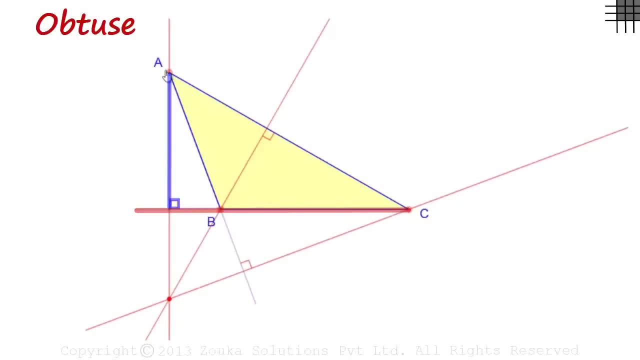 So this segment becomes the altitude from vertex A. Similarly, to drop an altitude from vertex C, We had to extend AB. After we draw all the altitudes, we had to extend AC, extend each one to form the orthocenter. This proves that in an obtuse triangle the orthocenter lies outside the triangle. 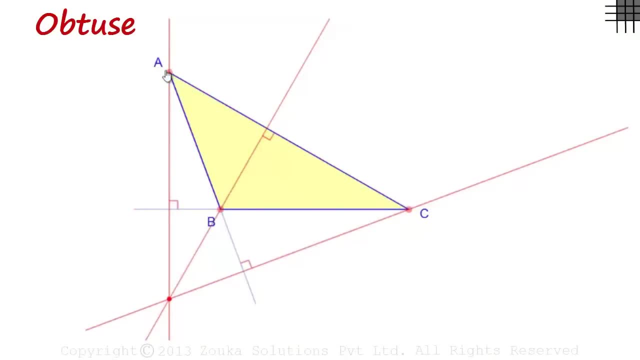 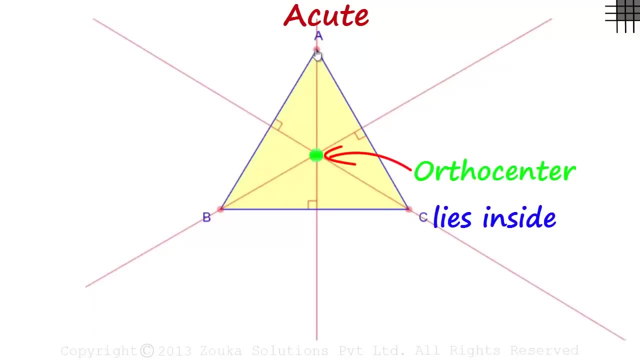 And the more obtuse the triangle gets, the further away the orthocenter will lie from the triangle. So if the triangle is acute, the orthocenter will lie inside the triangle. In the case of a right triangle, it will lie on the vertex. 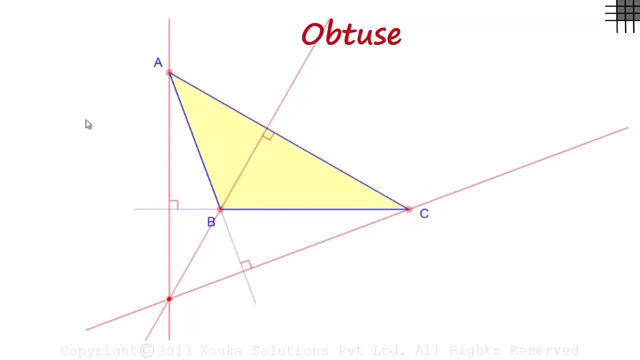 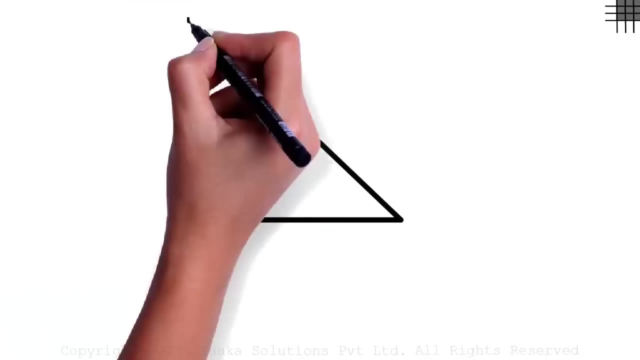 at which the triangle is right angled And if obtuse, it will lie outside the triangle. Let's understand this again: This is a right triangle. ABC. AB is the altitude from vertex A onto side BC. CB is the altitude from vertex C onto side AB.